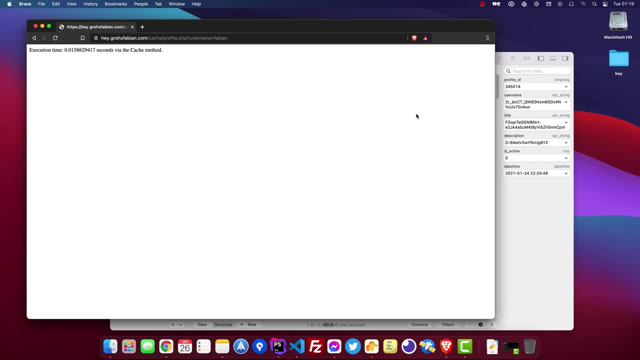 video. i'm going to show you exactly how i did it, with a real world example broken down into few snippets of code. you've probably heard of cache and the caching term before. it is the process of storing data into a temporary location for faster access. i've also written a detailed blog post. 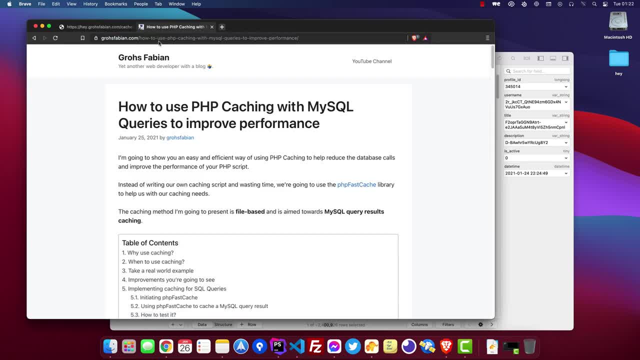 about this on my blog. so if you go to this link on grossfabiancom, i will make sure to leave a link in the description below. now let's talk about when and why you should use caching. keep in mind this highly depends on your situation and there is no definite answer that can apply to everyone. 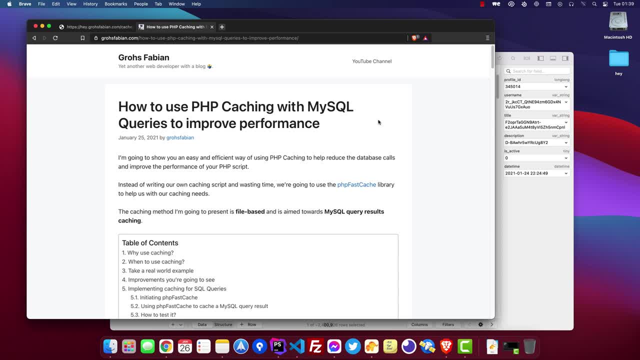 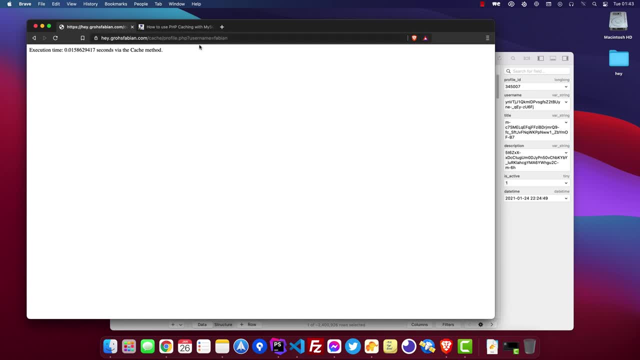 as everyone's project is quite different. now let me show you an example of where using cache is the right choice. we're back to this simple profilephp script that i've made that takes only one parameter, which is the username, and we're going back to the database, where you can see the 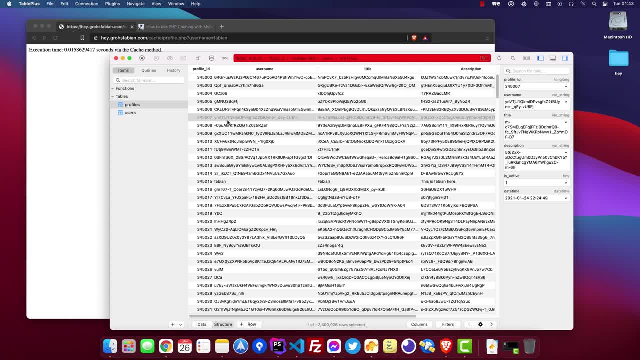 profiles table. this can be considered a very, very basic social media platform where people would access this profile link and they will want to see the title and description of your profile. now think about the fact that this profile can be accessed 100 times a day, 10 000 times. 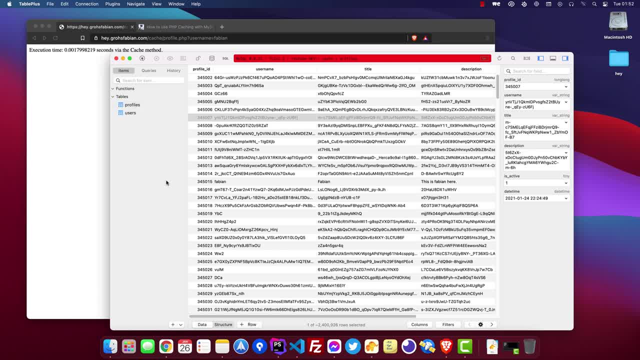 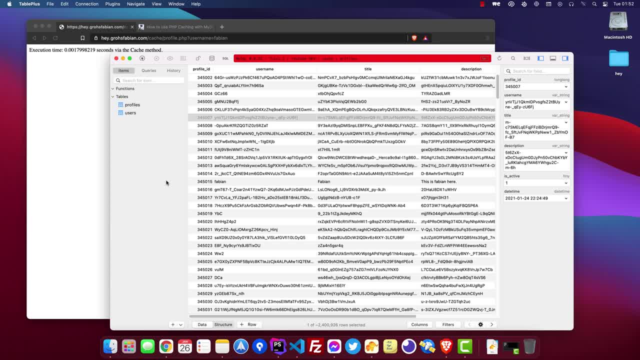 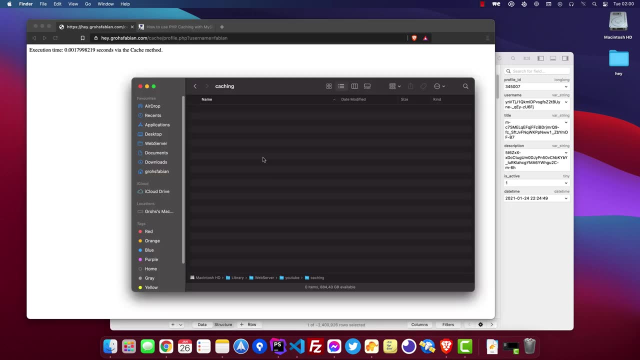 to the server resources than to read from a simple text file containing data from your server. why would you want to run the same query over and over again if you know that the data that you're going to return is the same? now, enough with the talking, let's go into the actual coding. so, as you can see, 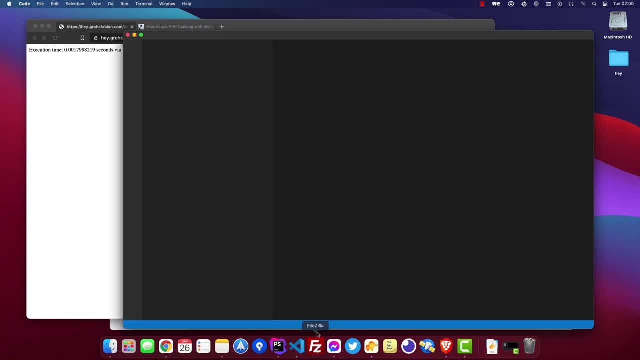 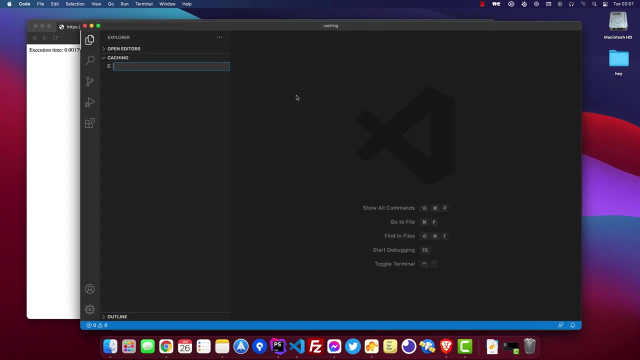 i have an empty folder right here. i will open it with visual studio code, because it's a free and pretty nice editor, and right here i will create an indexphp file which we're not going to use, and then i'm going to create initphp file in here. i want to initialize my database. 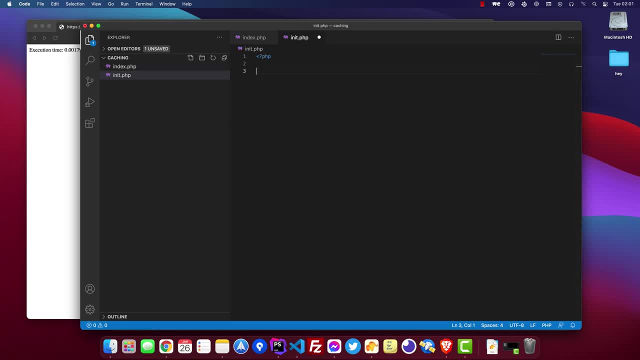 connection credentials for the database and also the caching library that we're going to use. for now it's empty, and then i will create another file. let's call it database credentials dot php. and now in here, i'm going to paste this code right here so that you can fill this for yourself, because i will fill. 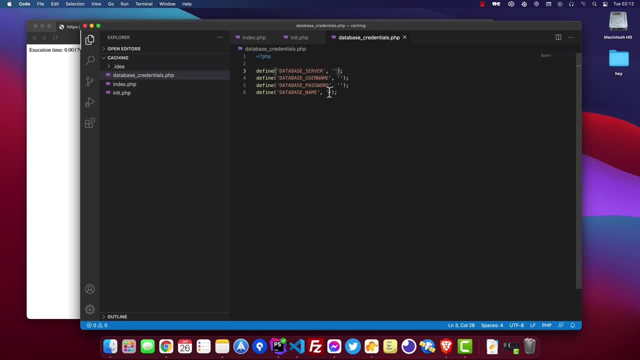 it with my database server username, password and the actual database name that you're going to use. so i will close this for now and then go right back to init and let's start with a database connection- database equals new mysqli- and then we're going to enter database server database. 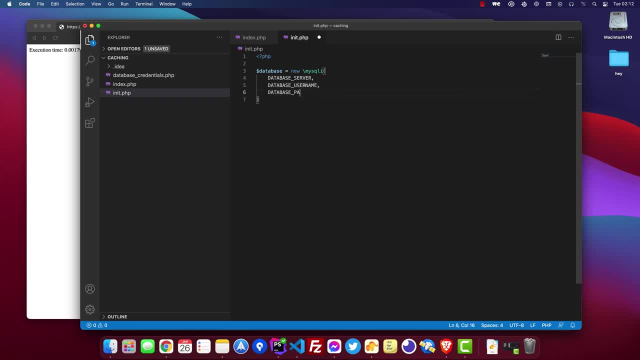 username, database password, database name. okay, we also need to import this. so we're going to require once and i'm going to require database credentialsphp. now, what i want to do is check if we have any database errors, connect error- and then we're going to die with this exact error, just so that we can see if there. 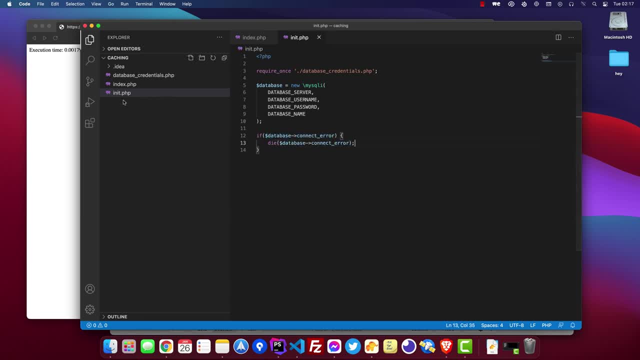 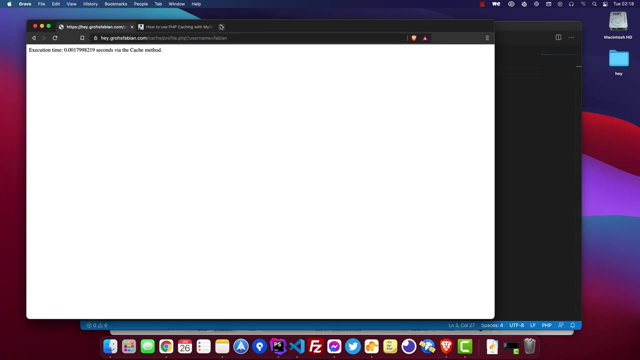 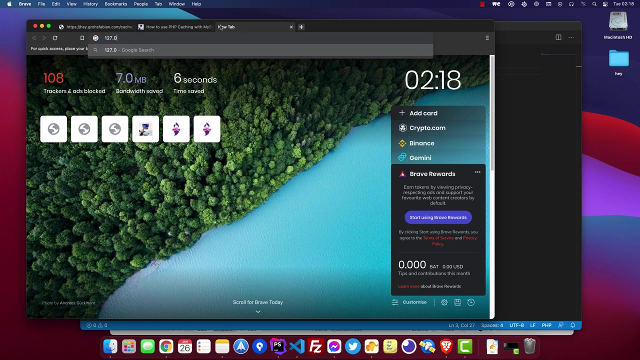 is any. okay, i will save the code and then i will go right back to the indexphp file and then i will require once initphp. okay, and now i'm going to go to the browser and i'm going to assume that your server, your php, your mysql and everything else is properly set up already. 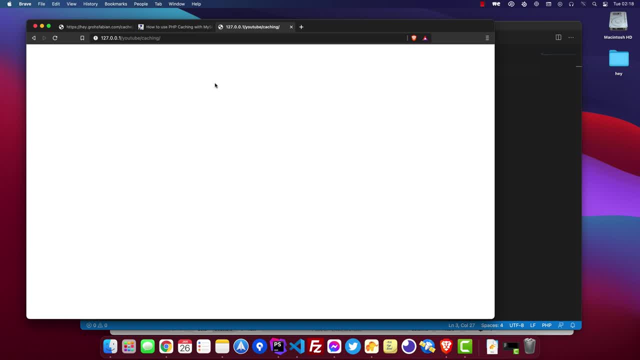 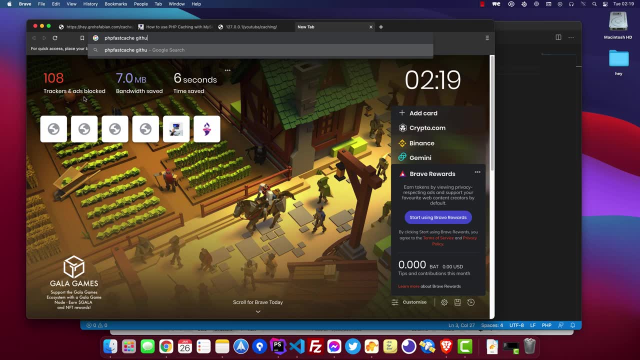 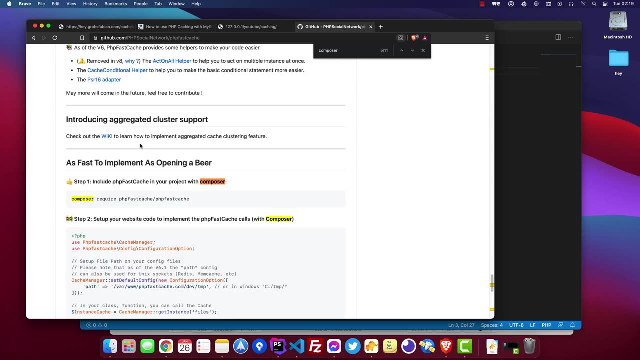 as you can see, we have no error, which means the database connection is working properly. now what i want to do is search for php fast cache, github, and i will go right here to the github page. i will search for composer and right here i'm going to copy this, paste it right here. 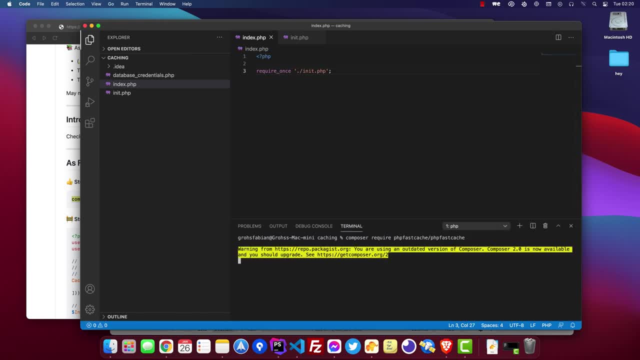 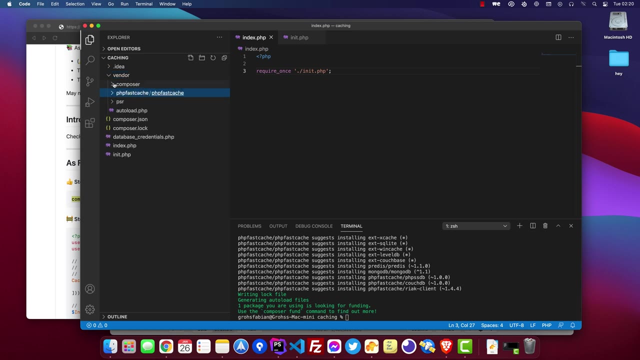 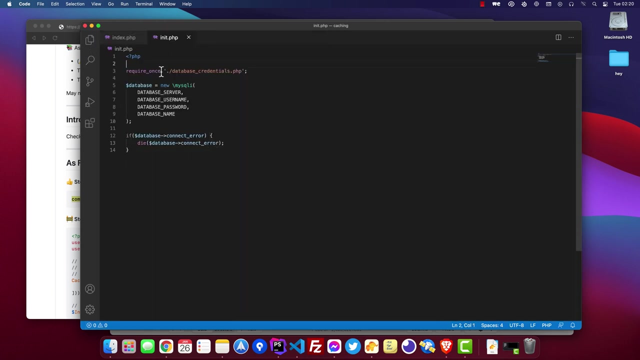 into the terminal and this is basically going to load the library directly into this folder. again, you'll need to have composer already installed. as you can see, this created the vendor folder which contains the php fast cache library. we're going to go back to init. i'm going to close all this up and right here. i just want to say require. 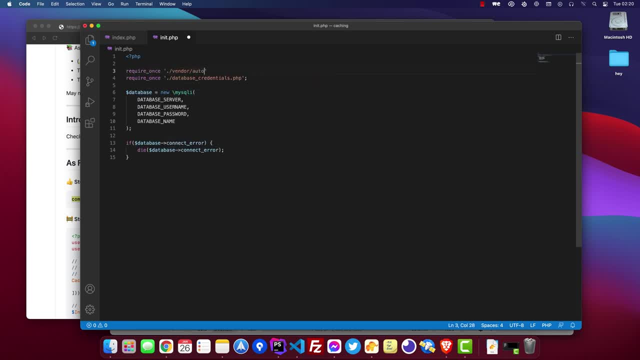 once, and then vendor autoloadphp. this will make sure that the library is loaded so that we can use it. okay, now let's go back right here and create a new file. i'm going to say profilephp. okay, and what i want to do right now is initiate a profile username variable which will basically: 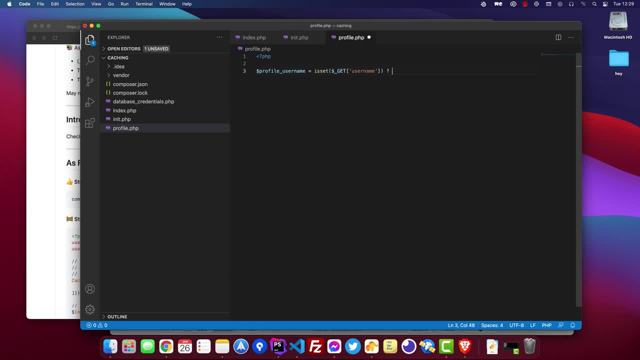 check for the get username query parameter to make sure it's set, and then i'm going to use escape string function on get username. else we have no, if not profile username. i'm just going to die and say profile username specified. of course this is just for testing purposes. and right now what i want to 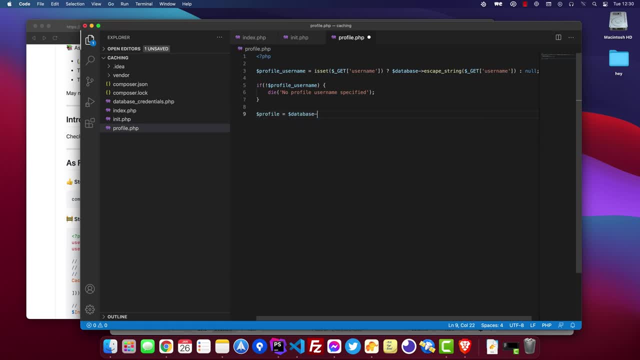 do is get my profile data, which is going to be as easy as this: select all the data from profiles table where username equals, and i will put the variable of the profile username right here, just like this. and then i'm going to go with fetch object and that would be it. let's see, i'm going to print our the profile. 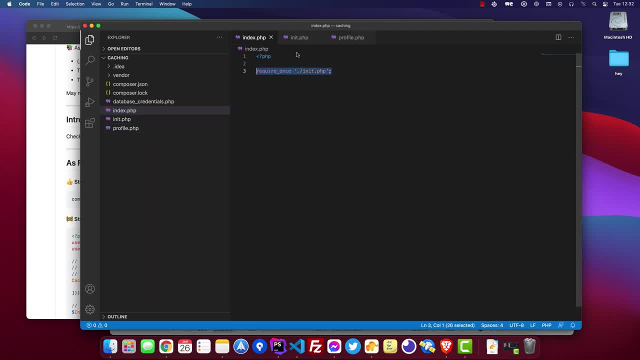 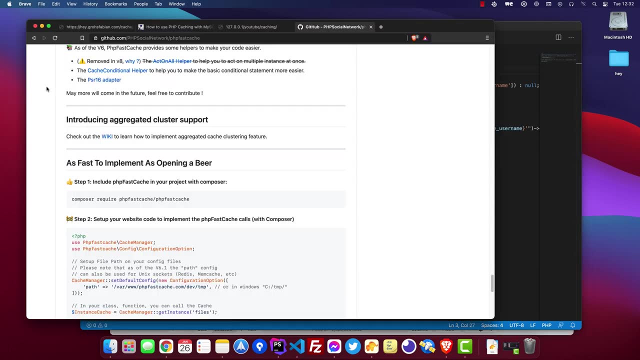 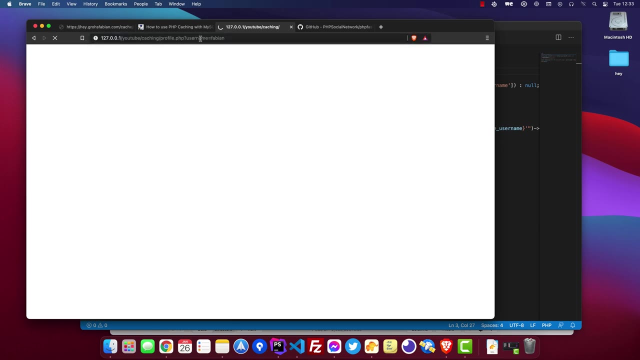 and of course we actually need to go back to the index and copy this line of code, because we need to have the database initialized. and then i will save this up and let's go right here. go to profilephp- username, and i will specify fabian and of course it's searching through. 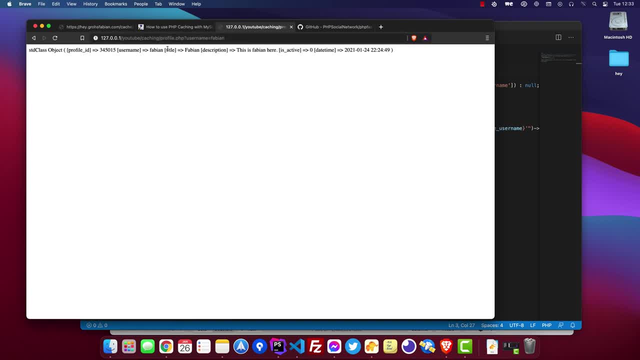 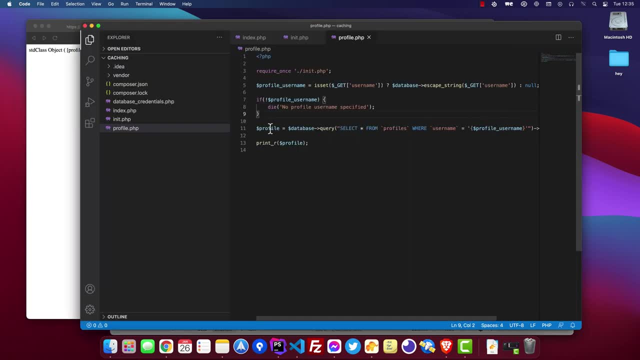 two million and a half rows from the database. and there you go. this is the profile, and right now, what we want to do is being able to cache these results of the profile query. what i'm going to do is go to the initphp file and i'm going to start to initiate the cache configuration. 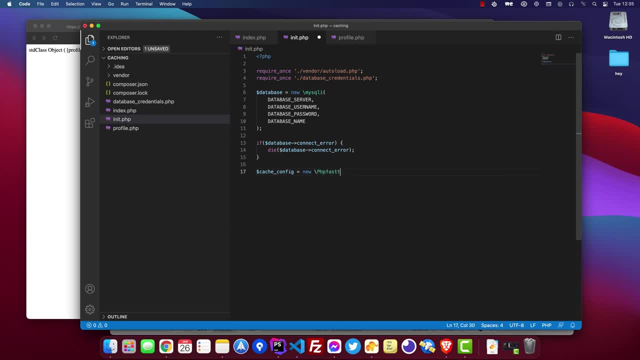 right here i'm going to say: new php fast cache drivers. i want the file driver. and then i'm going to say config file drivers. and then i'm going to say config file drivers. and then i'm going to say config. right here i'm going to input all my configuration. this is already set by me. 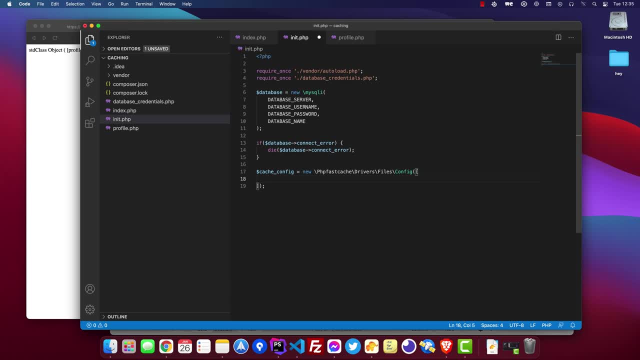 these are my preferences. if you need anything else, you should go and look for the documentation on github. there are plenty of options for this library, and what i want to say right here is the path. the path is going to be used to store these text cache files with the data that we're going. 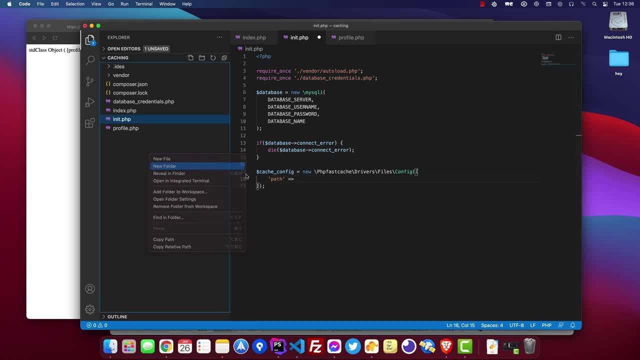 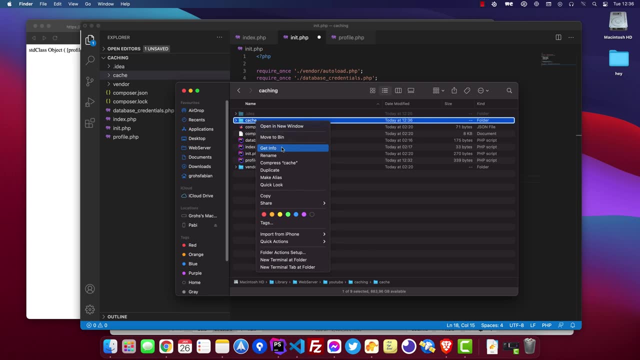 to input. so i'm going to also create right here a new folder which is cache, and then i will go back to the finder, make sure this has a ch mod 777, so that the script has access to it and has writing permissions. and then i'm going to go right here and specify it as: 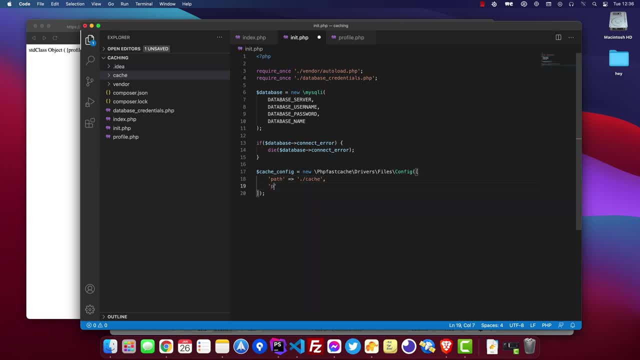 cache okay. next one is prevent cache slams, and i will set this to true cache slams, timeout 20 and also secure file manipulation through. now what are these lines? these lines help prevent the cache from being generated multiple times and colliding with each other if the same resource. 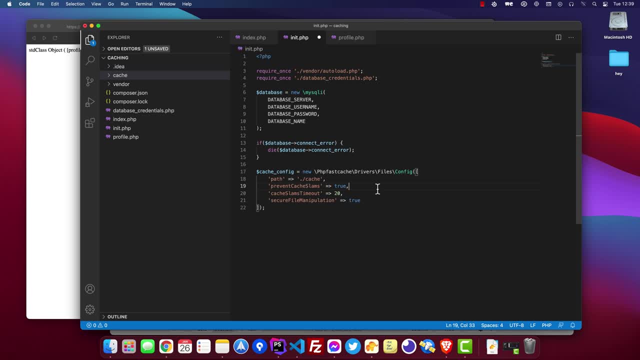 is requested at the same time while the cache is being generated. it is an extra security layer which i would definitely suggest for you to use right away. i'm going to initiate php fast cache cache manager, set default config, and i'm going to pass in the cache config we just created. 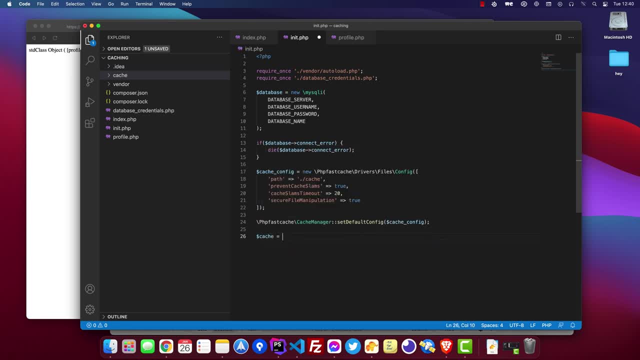 right now i'm going to initiate another variable named cache and i'm going to say: php fast cache cache manager, and then i will get an instance for the files cache system. all right, now, let's test this out, and i'm going to go in the browser. all right so. 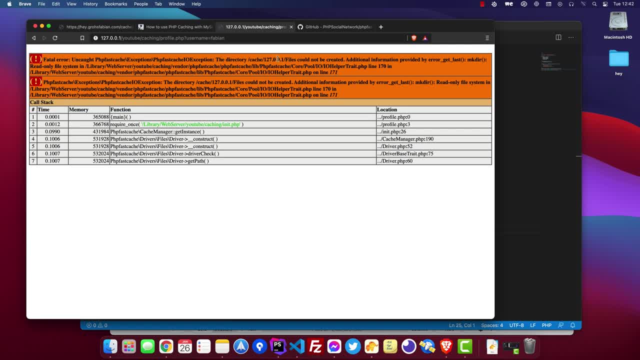 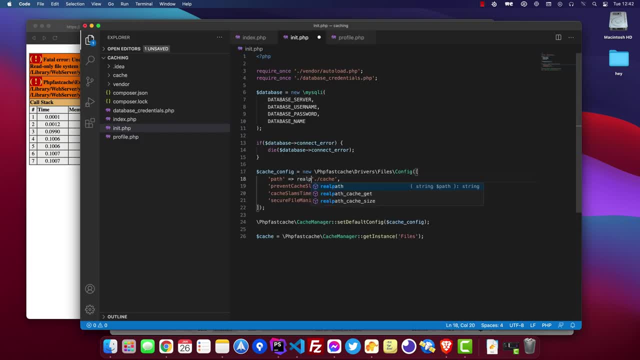 it seems that we have a problem. the directory cache- okay, files could not be created. all right, let's go back in the initphp file and i'm going to say, right here, real path there, and then i will do this. this just makes sure that we have the correct path. 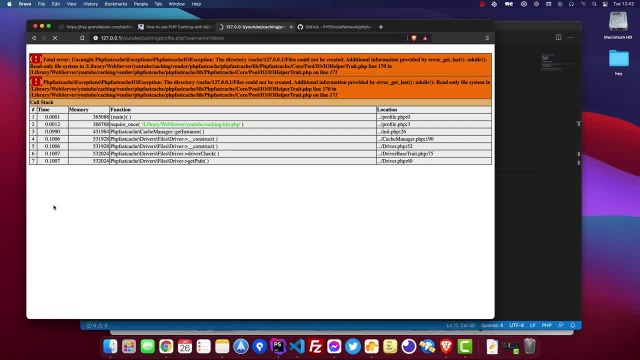 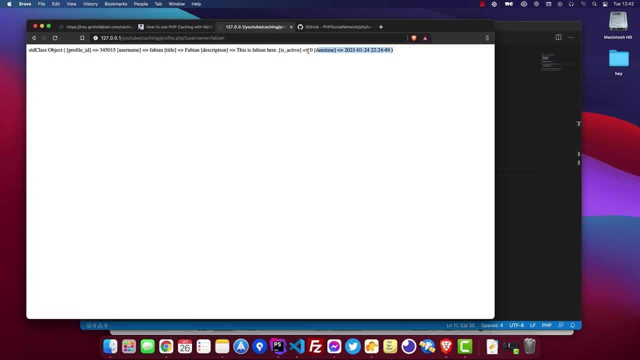 and i will save it. let's go in the browser, hit refresh, and it seems that it's working because the query is processing. okay, let's go back in the browser, hit refresh, and it seems that it's working because the query is processing. okay, keep in mind, right now we only have the cache initialized. we don't actually make use of it. 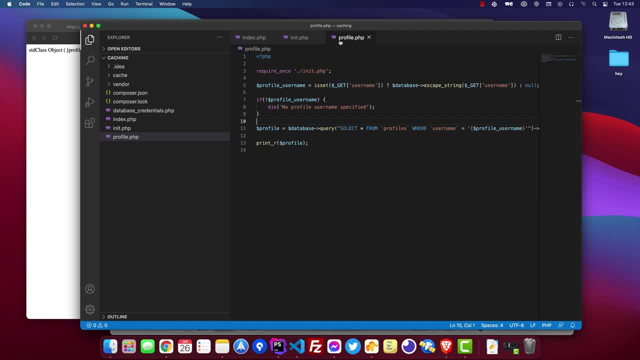 and right now what we want to do is start to use the actual caching. so go back to profilephp and right here i'm going to say cache instance and i'm going to use the cache variable that we just initialized, and i'm going to say get item and here you will need to specify the key of the cache. 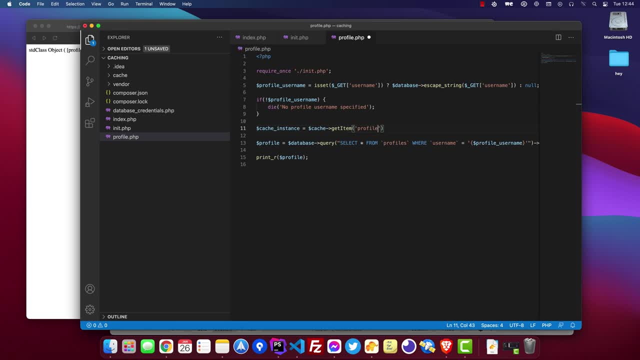 so i could do something like this profile, but keep in mind, this profile data is dynamic, so i'm going to give it a dynamic name, such as profile, question mark username and i'm going to say profile username right here. what we want to do is check if this actual cache exists and is not expired. if is no cache instance. 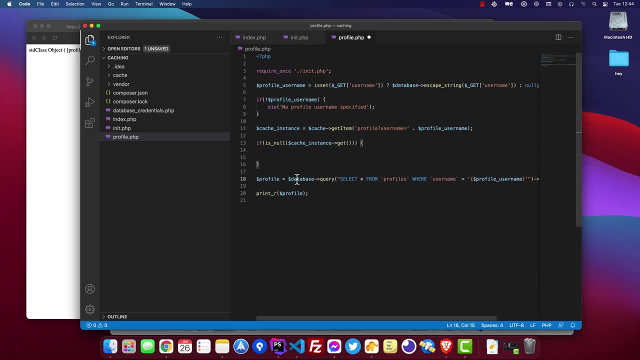 get, then what we want to do is actually run this query and right now, if we want to run this query, we're going to save this data that we have in this profile variable into the cache. we use the cache instant, we set the data for this variable to profile and then we're going to mention expires. 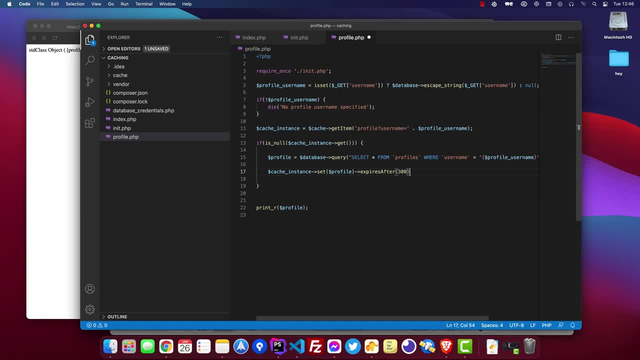 after 300 seconds, for example, five minutes- then we want to use the main cache variable and then i'm going to save it and then right here i'm going to have the else function in case the cache already exists. so i'm going to get with profile and then i will say: 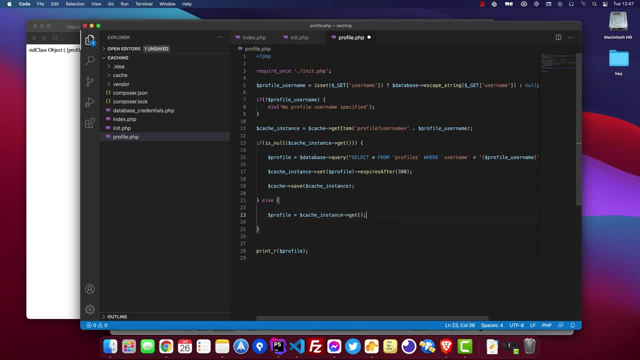 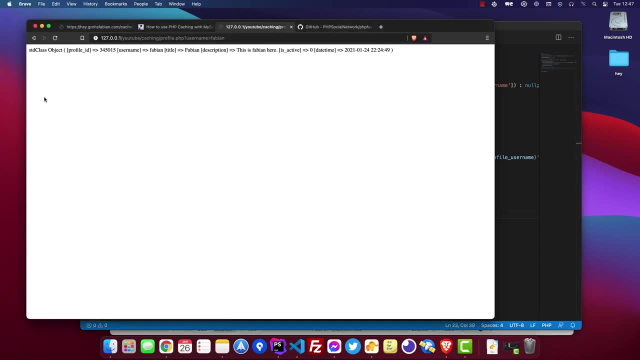 cache instance get. what this function does is basically return the data that you've saved to the cache. i'm going to hit save and right here, i'm going to hit refresh. the first request is going to be from the database and the second request should be as fast as possible. hit refresh. 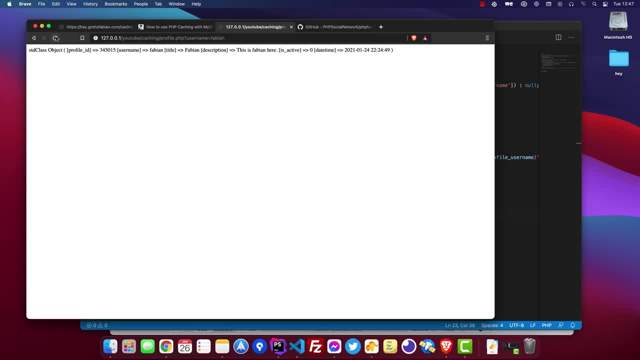 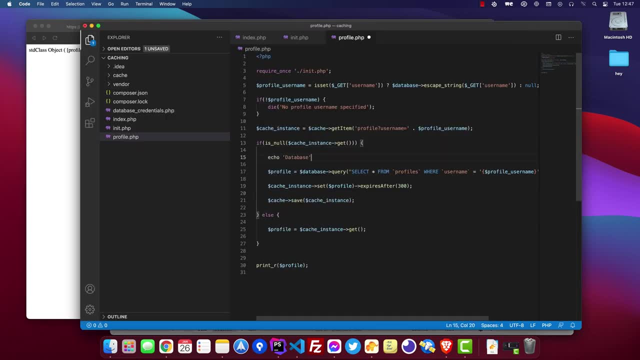 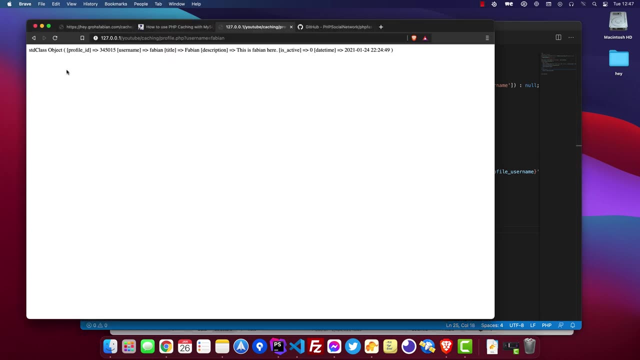 again and, as you can see, it's instant. right now this data is returned from the cache. let's test this out. i will say right here, echo database and right here i'm going to say echo cache. if we refresh right now, you're going to see cache right here, because the data is returned from. 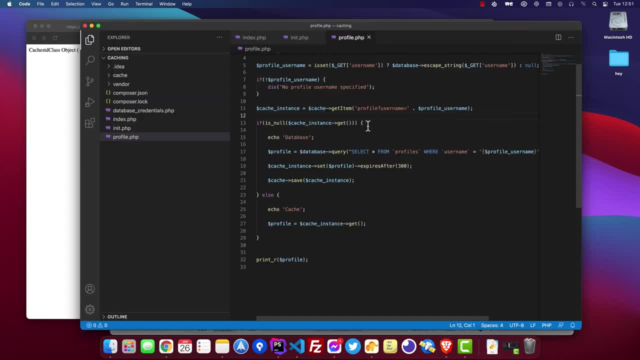 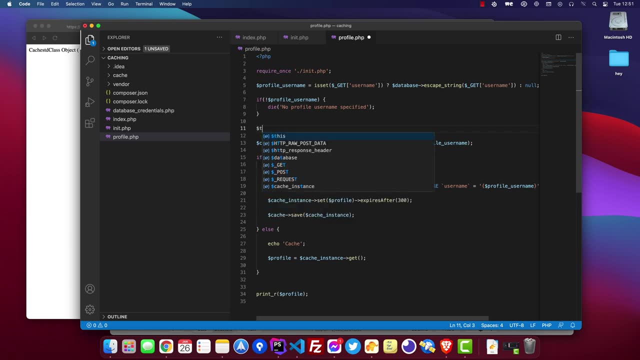 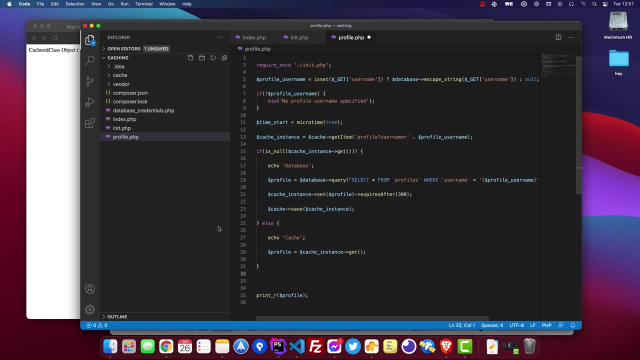 the file system now how much faster. exactly what i'm going to do right here is set a new timer so that we can see the execution time of this snippet of code. time start: micro time, and i'm going to set the float to true. and below this snippet of code, i'm going to paste another snippet which will: 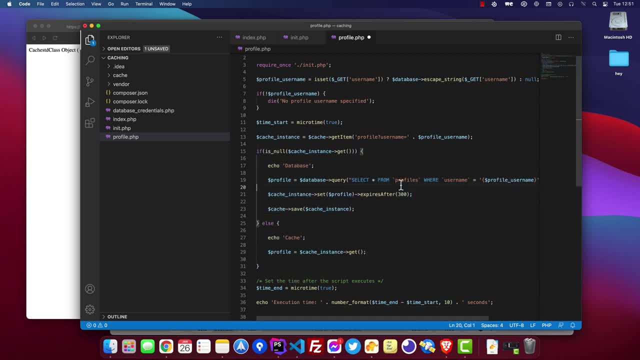 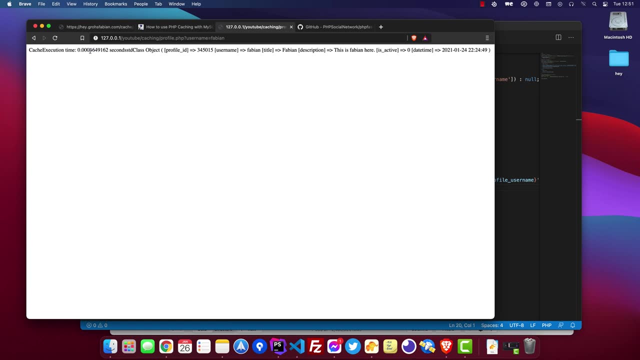 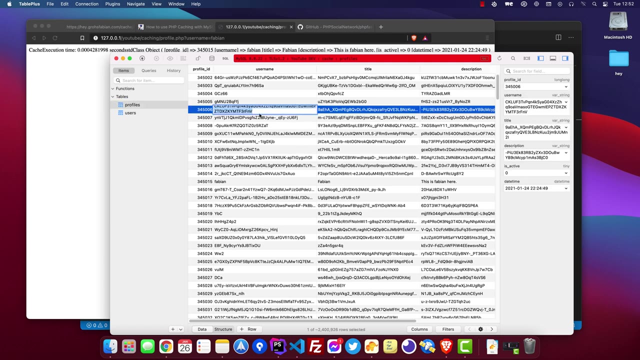 calculate the execution time of this code. so i'm going to save refresh and, as you can see, 0.000504 right now. let's try to search for another profile. i'm going to go in the database and i will copy this username, which is again a randomly generated one, just for testing purposes. 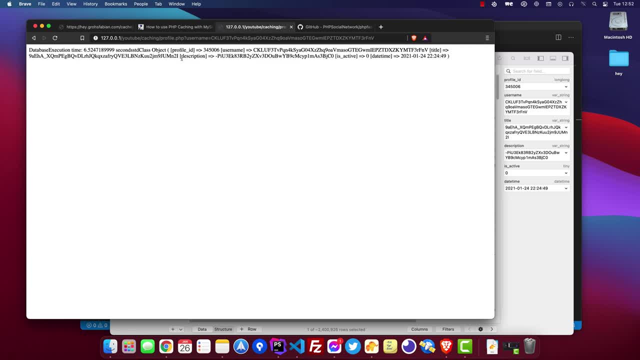 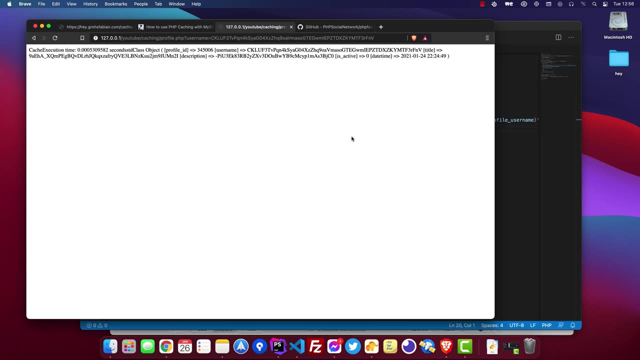 i will search for it right now. and right now you can see it took about 6.5 seconds for this query to execute. now, if we hit refresh again, it's cached and it's instant. now i want to make some extra points on this subject. if you're going to use this in a production setup, where you would also have 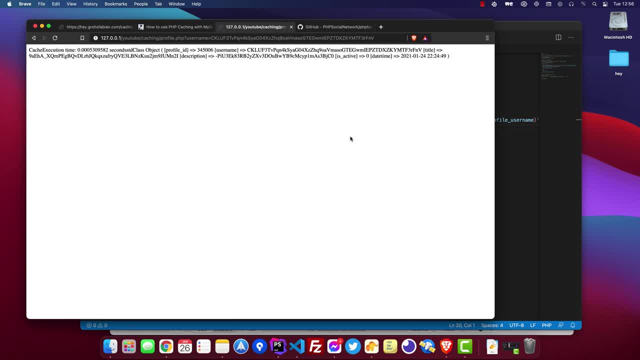 the ability to delete the user or change his details. you don't want to show the user outdated details from the cache. once the user changes his details, the cache for this user should be deleted. how you can do that? it's pretty easy. i will just show you the command right here in order to delete this cache. we can do the. 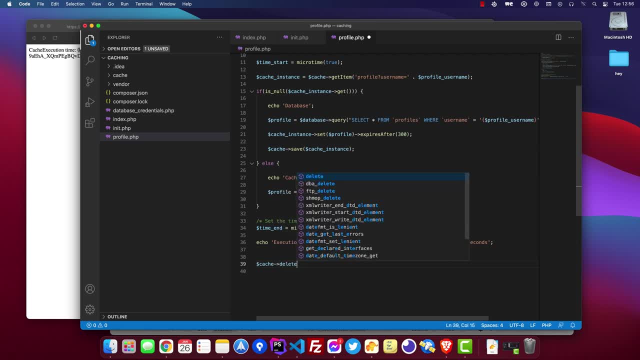 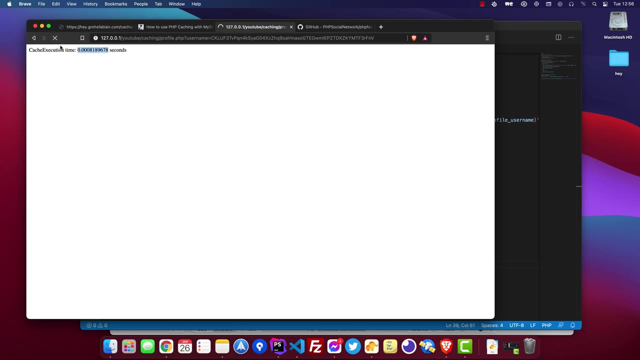 following: i'm going to say cache delete item and i'm just going to specify the key of this cache, which is the same one. i'm going to hit save. and right now, if we reload, the first reload is from the cache and the next one would be from the database, because we just reset it at the bottom. as you can see, it took.